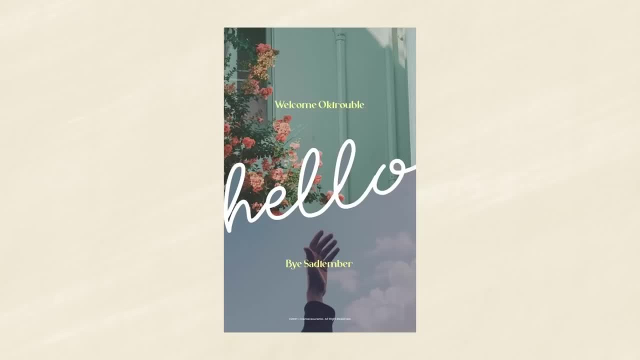 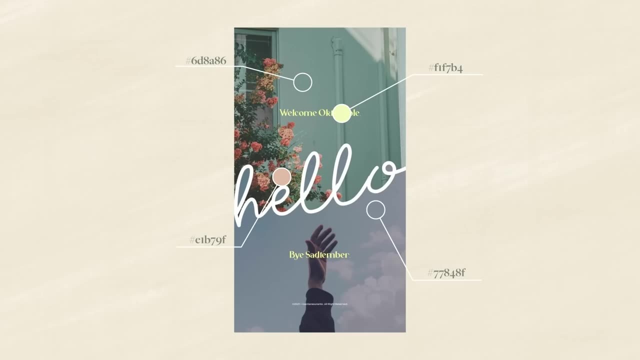 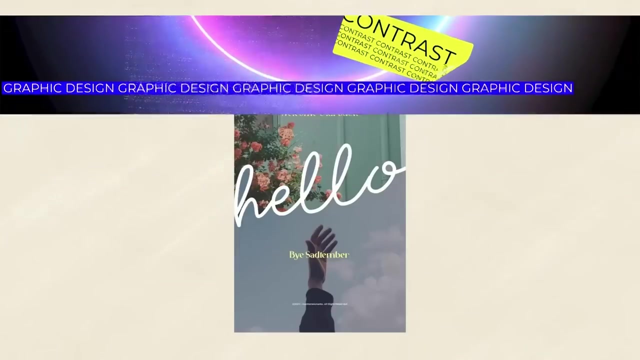 integrate emotion into your designs. But on this design, firstly, the colors used are desaturated and muted. Washed out, pastel and desaturated colors automatically appear more calming. Contrast that with the vibrant lime green on the other design, which is energetic. Also on this floral design, we have well. 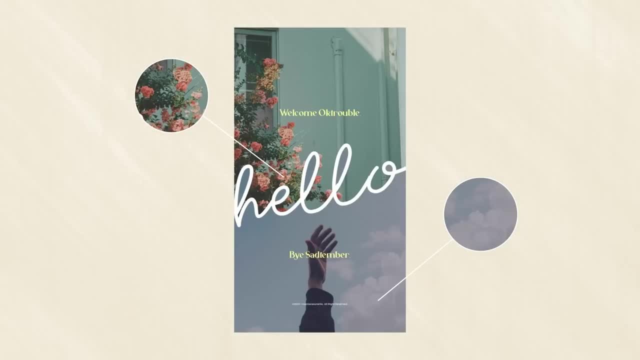 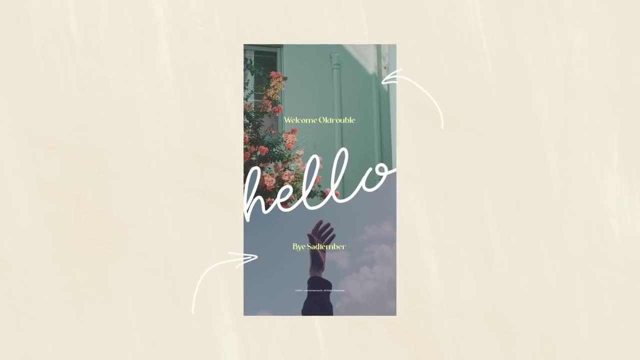 colors and nature. This kind of imagery is automatically peaceful and calming because it triggers the nature side of emotion. There is a lot of open white space on this design as well, which allows everything to breathe and to have peace on the design itself. And then also we have 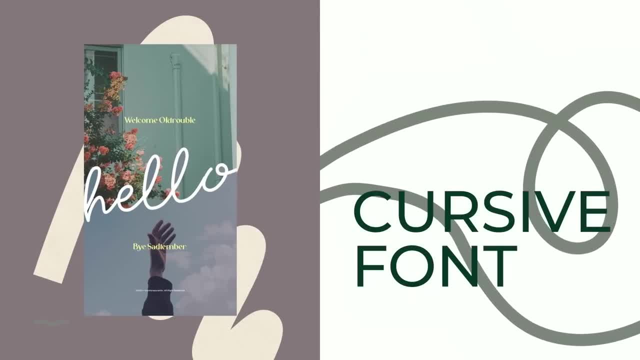 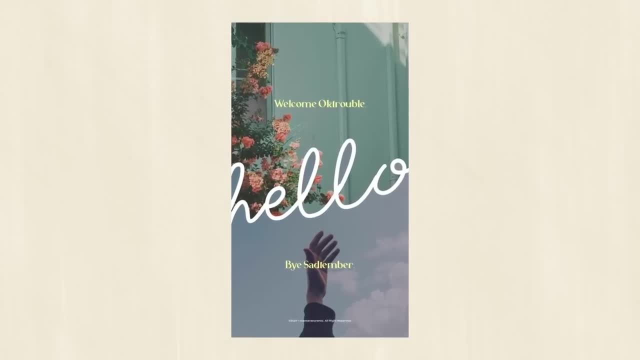 that freehand cursive font on the word hello, and this is very organic and very personal and that just adds to the more peaceful nature. And so, as you can see, each aspect of this design can be linked back to emotion in some way, shape or form. 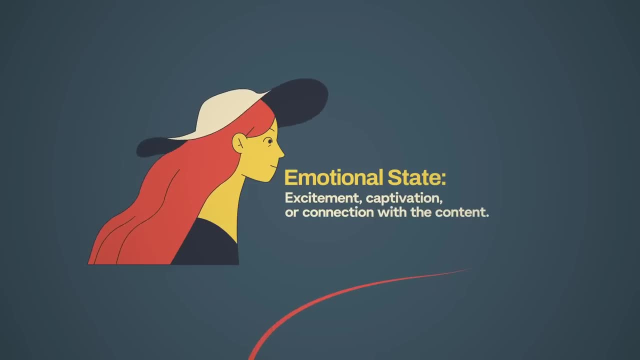 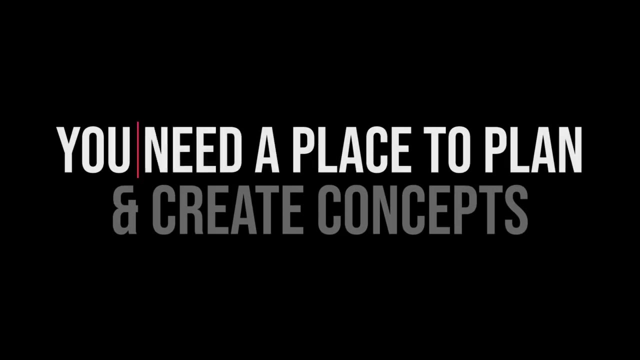 If it's a typography, the color, the imagery, whatever it is, it's all emotional based. It is a great start to actually understand how important emotion is in graphic design theory, but you also need to plan out a design and have a place to create concepts and ideas with emotion. 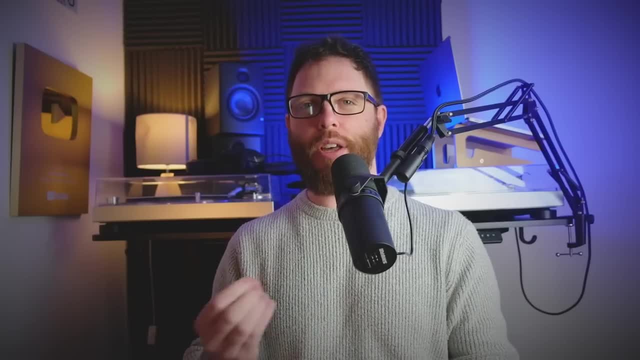 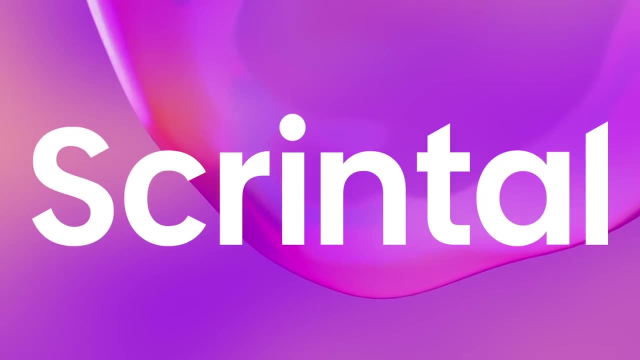 in mind. There is an app that actually really helps when working through graphic design theory, like in today's video, and it also helps me work through graphic design briefs really, really easily, And that app is Screentool. So here's the project board for a Surrealist Nike poster design that I 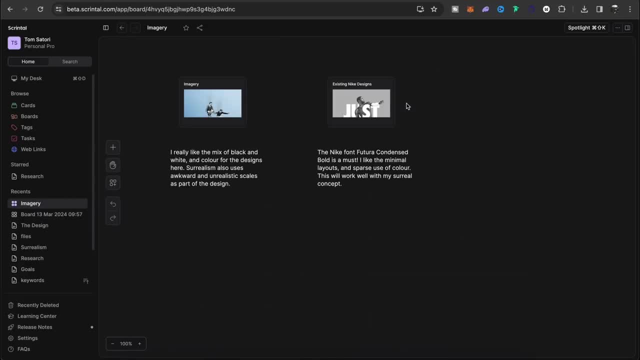 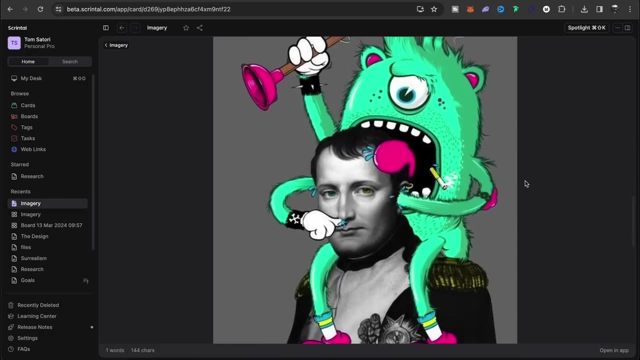 on for a past video. Scrinter is a really great way to structure your ideas and your thought processes when working on a project. For example, up here in the research section, I've compiled some surrealist designs for inspiration and I made a few notes on them in relation to my concept ideas. 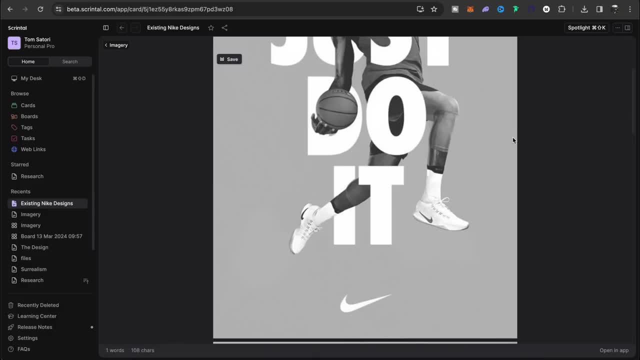 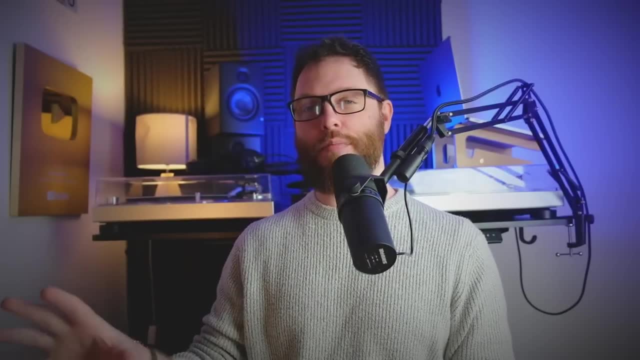 Also here I just compiled some existing Nike designs so I can actually make sure my design was on brand when working on this Nike project. Keeping a design on brand when working for a specific brand is really, really important and any project has goals and, as you can see here, one of 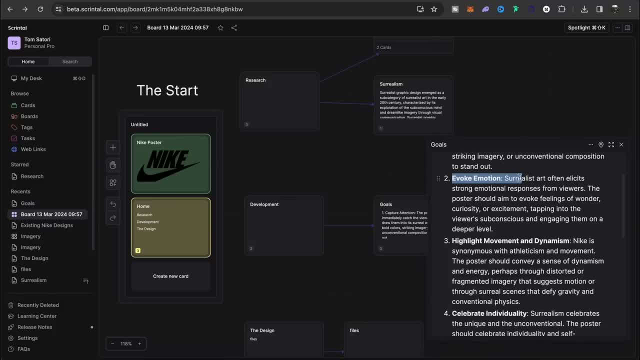 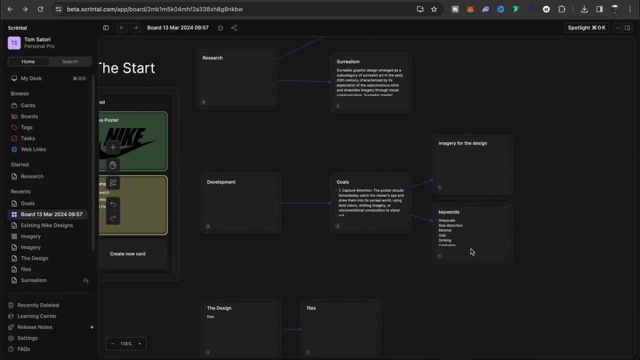 the main goals for my surrealist design was to tap into emotion, like we've been talking about in today's video, and from that emotion I generated some keywords that would actually help me in the design's creation, and in the end the design turned out pretty dope, if I do say so myself. 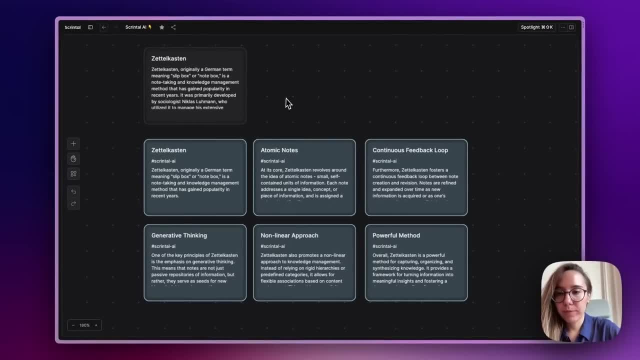 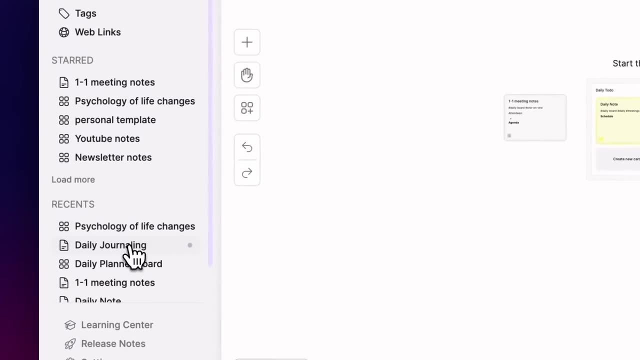 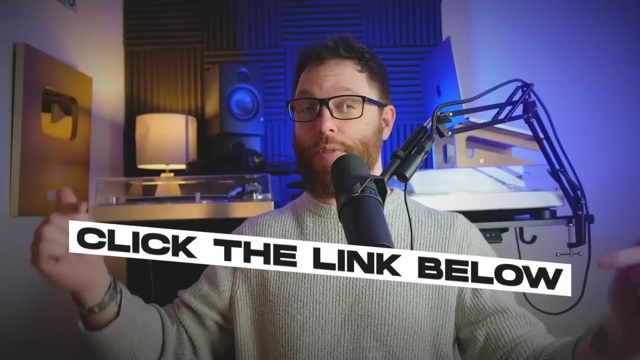 Scrinter isn't just for planning out projects like this. it's also good for note-taking, goal setting in general, storytelling and managing your project. It's just a really neat and a really intuitive way to remain productive in whatever you do, and you can grab a 10% discount on Scrinter when you use my link in the description box below and. 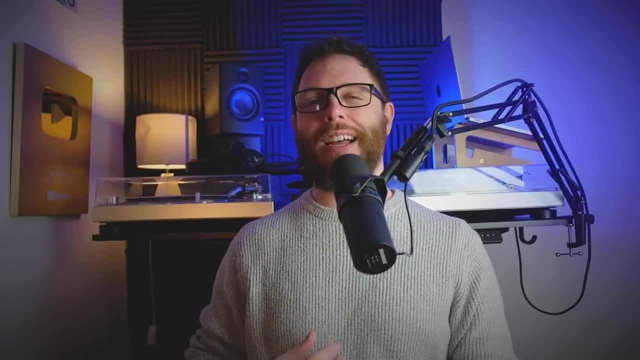 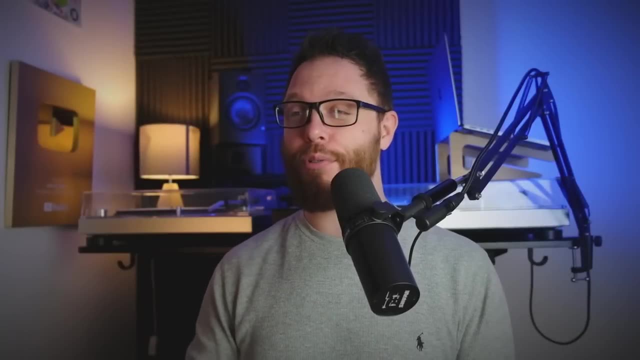 that discount is valid for four weeks after the publication of today's video, and so thanks to Scrinter for keeping me productive and also for sponsoring today's video. Right now, we're going to look at a system that you can use on any project and work through to implement emotion. 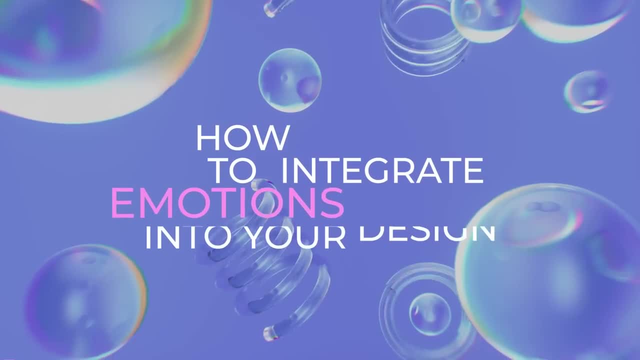 in really, really useful ways. This process has three simple steps, and the first step is to identify the right emotion for your project. The first step is to identify the right emotion for your project and identify the emotions you want to evoke on your design, and to do this just simply. 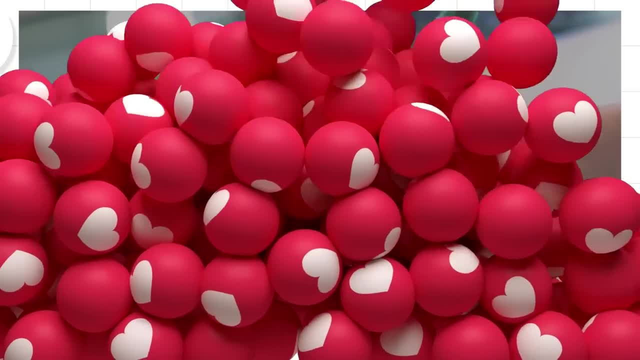 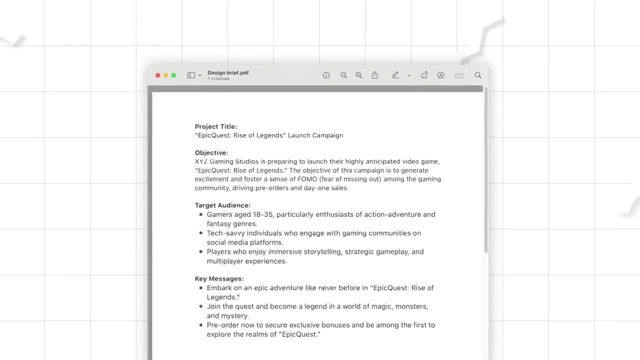 take your design brief and then gauge what emotions you want the audience to feel from the design brief and to show you how that works, let's take this video game poster design brief as an example. A lot of designers will look at this and they're going to miss the crucial key points on. 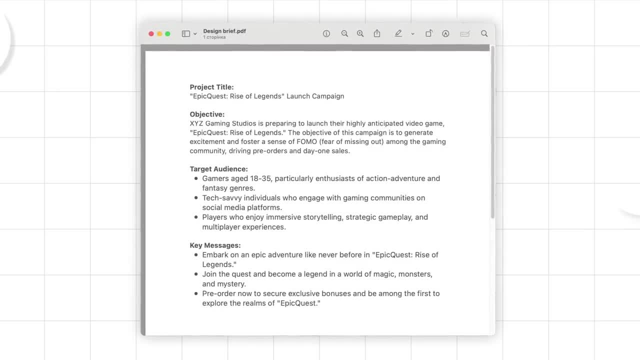 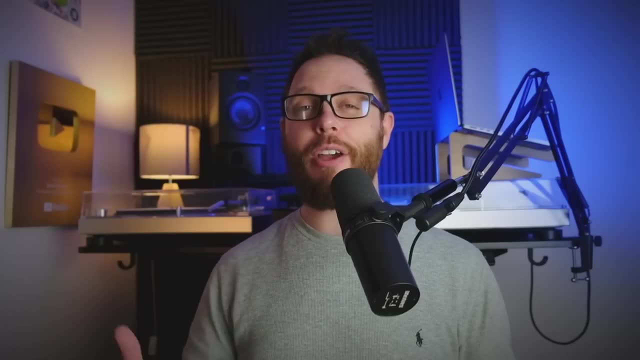 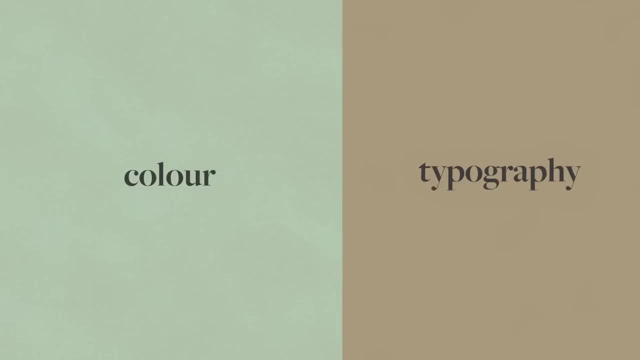 this brief the emotions Notice in the brief. it says excitement and also FOMO or fear of missing out. These two golden nuggets of information are what we're looking for in a design brief. First step is to write down somewhere four categories of color, typography, imagery and 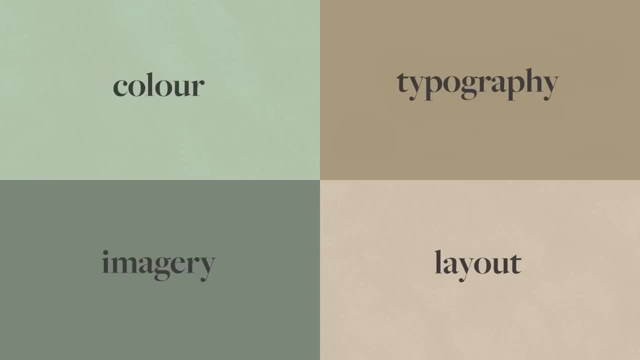 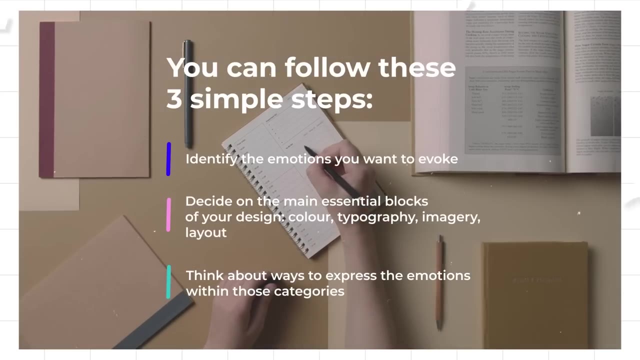 layouts. These are the main, essential building blocks of your design, or any design for that matter. The third step is to write down ways you can express the emotions within these four categories. So for color, you might want to use reds or possibly vibrant, bold colors. This is 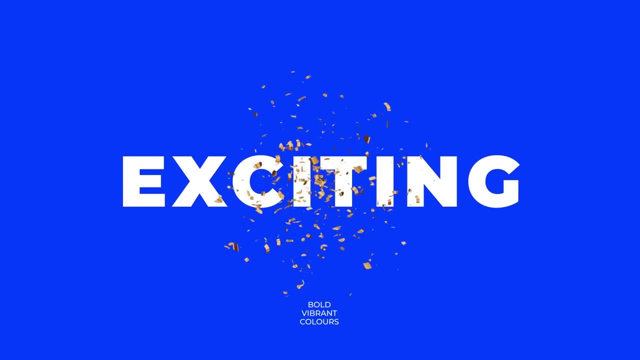 because these colors are hard-hitting and exciting, which leads back to that emotion of excitement. One of the first things that you want to write down for the design brief is strong emotions, For, For typography, we might want to go with futuristic, bold, sans serifs. 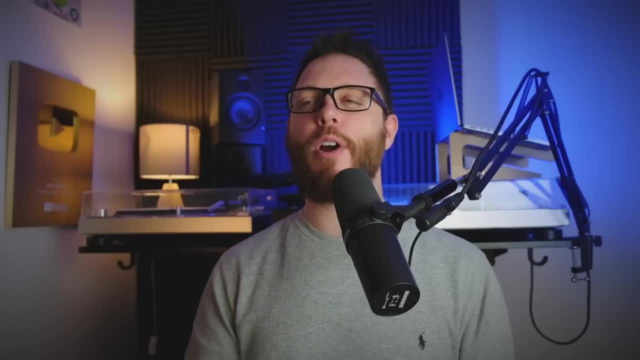 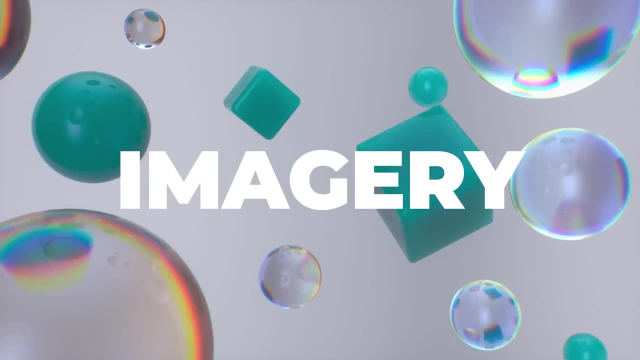 And that's again leading back to excitement. But what about the FOMO, or the fear of missing out part of this brief? Well, when it comes to imagery, we could maybe include a countdown timer on the poster, And this would make the audience feel like they don't have much time left to buy the game or to wait for it to launch. 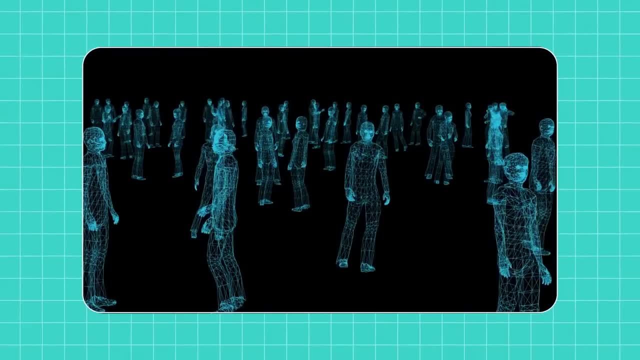 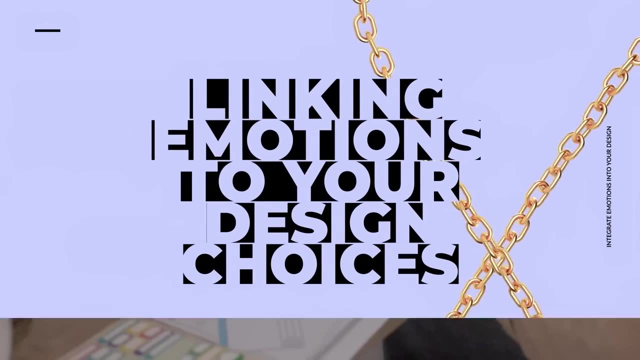 Or we could even make the poster look like it's a really crowded virtual world of many different players. See, it's simply about linking emotion to design choices And, yes, you will need to learn about the basics of things like different typefaces and how they evoke different psychological attributes. 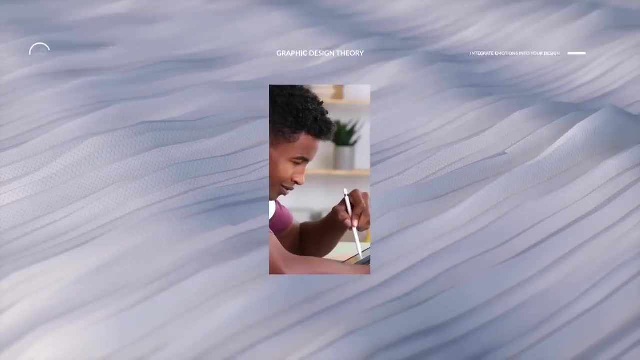 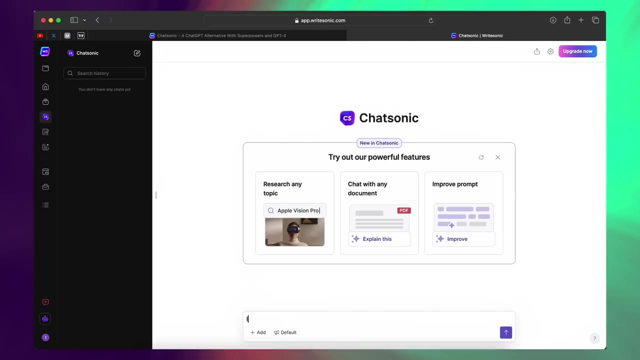 But stuff like that does come with experience. The emotion is the key factor or fabric of a design. However, there is a trick I've got up my sleeve that you will want to see Now. this is ChatSonic. It's kind of like ChatGPT, but some would say it's better. 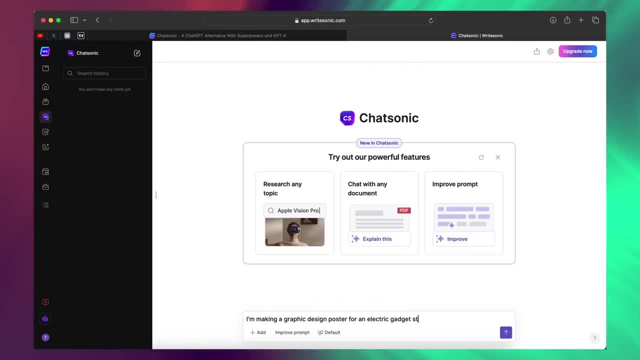 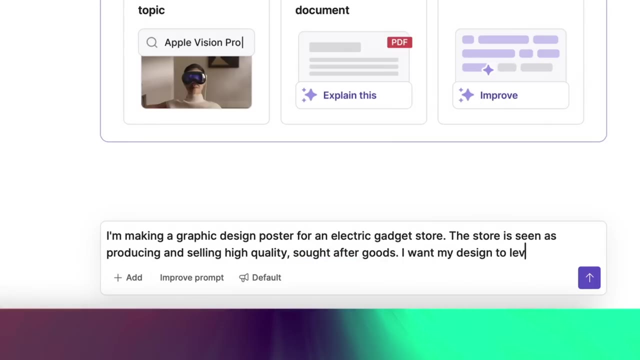 And hashtag, not sponsored. It could bring up articles and information all the way up to the present day, something ChatGPT cannot do, But for today's video. here's the trick that you can use for any design project using this thing. Now, here I'm explaining to the AI that I'm working on a poster design project for an electrical gadget store. 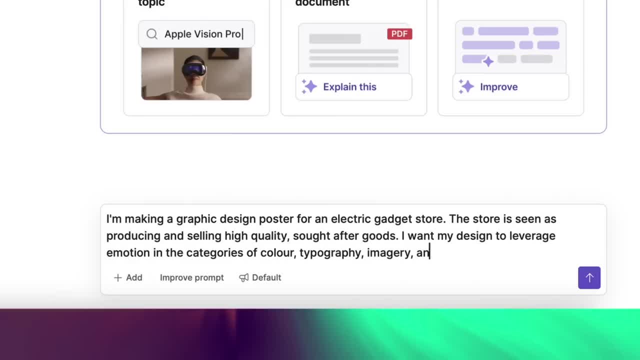 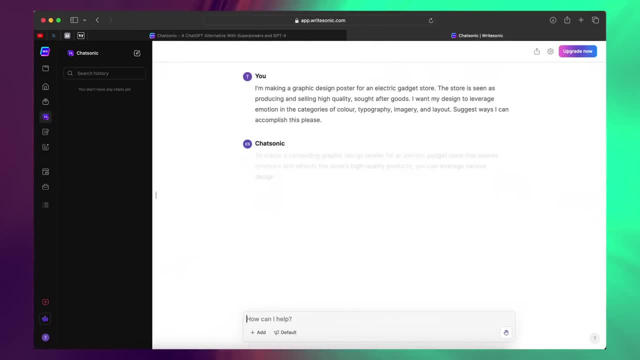 And, like we saw in today's video, I want to leverage emotion within those four categories of color, typography, imagery and layout. Now, ChatSonic is free, by the way, And as you can see here, It gives us some guidelines for the design in regard to those four categories. 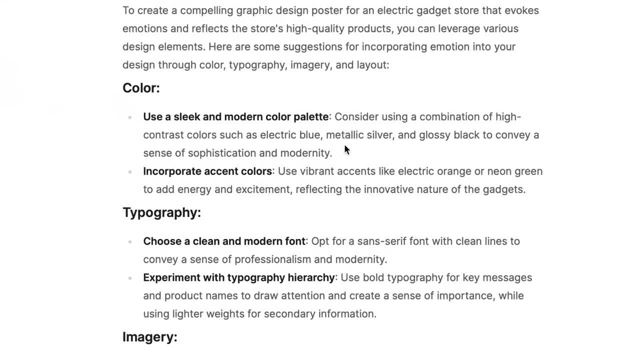 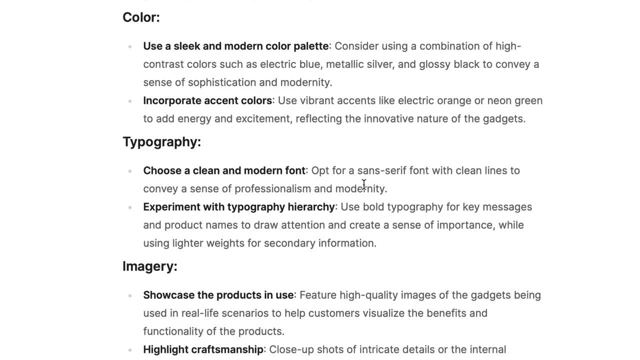 Now, importantly, as you can see, it explains every single suggestion and it backs it up with some theory. This is great for those who want to learn, but also it gives you ammunition in any design pitch to a client. It allows you to back up your reasoning and your design choices. 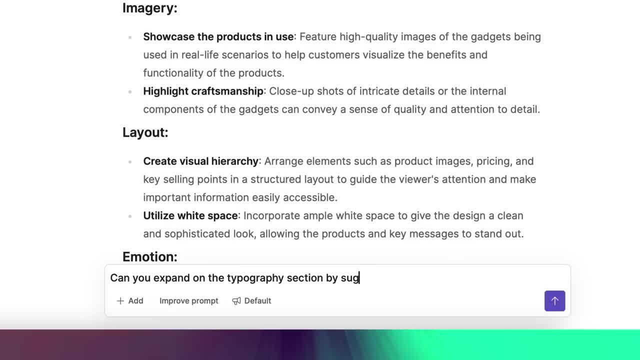 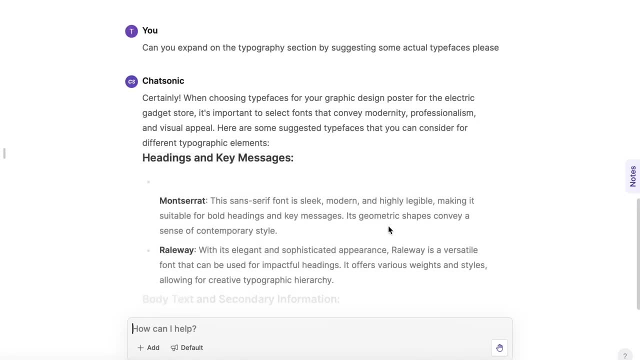 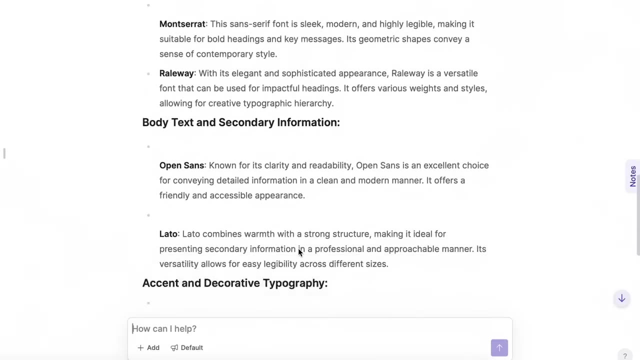 Now I can take things a step further and I can ask it to expand on the typography section and suggest some actual typefaces for my poster design, And with these results coming in, we can see some suggestions for headlines and key messages and then some typeface suggestions for the body text and so on. 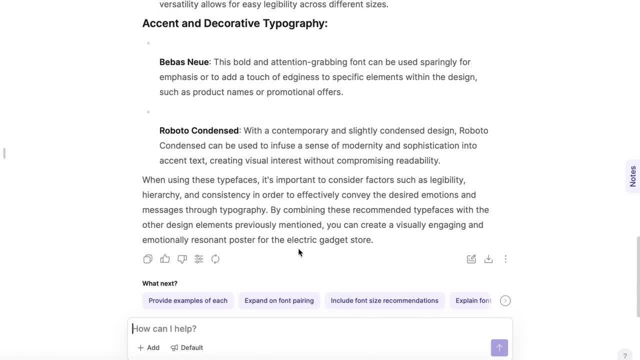 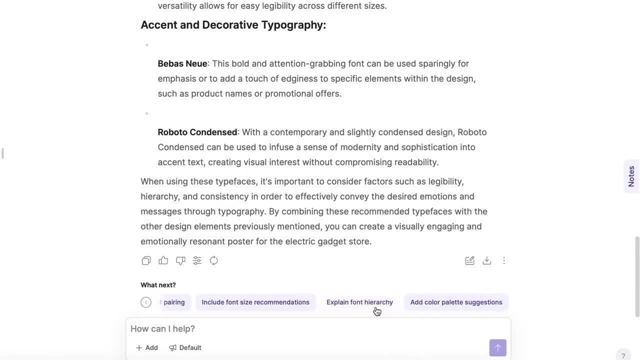 These suggestions should be considered and thought over by the designer rather than just blindly following them. Also at the bottom here, ChatSonic has other further suggestions that you might want to explore, For example, some color palette suggestions. Yeah, this tool is really cool. 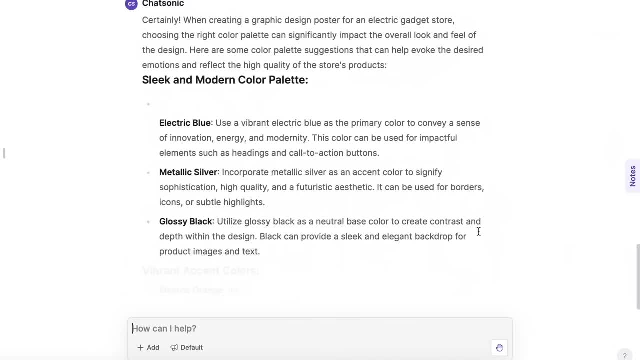 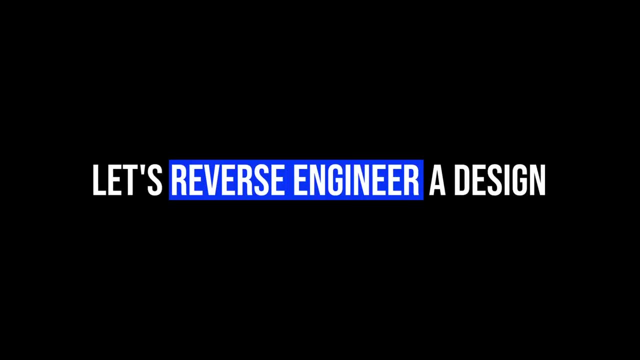 And again, I'm not sponsored by this. I just think it's a really cool tool. It's a really cool thing to use when working on design projects. Let's reverse engineer a design using that three-step system we looked at earlier, And this is just so you're very crystal clear on how to use it on your next project. 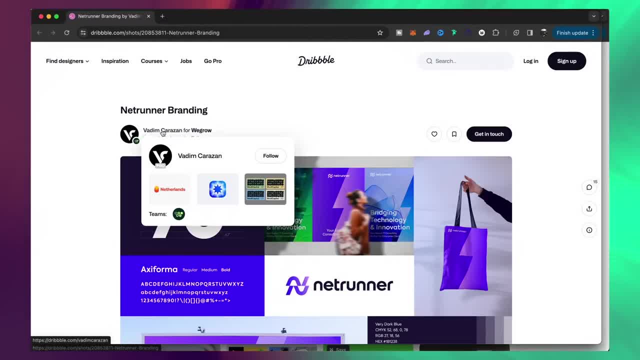 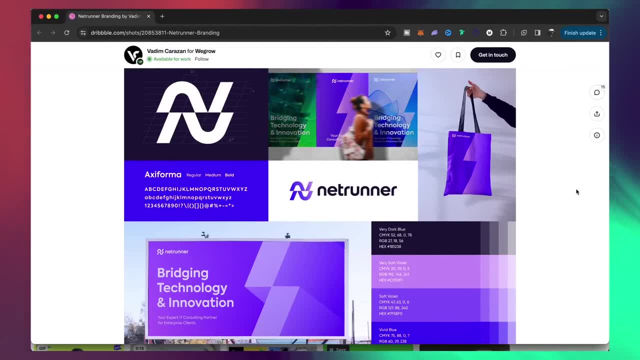 So we have a branding project by Vadim Karazhan, and that is Netrunner. Now, I do love this branding project And, before we reverse engineer it as I briefly scroll through the project, think about everything we spoke about in today's video in regard to emotion. 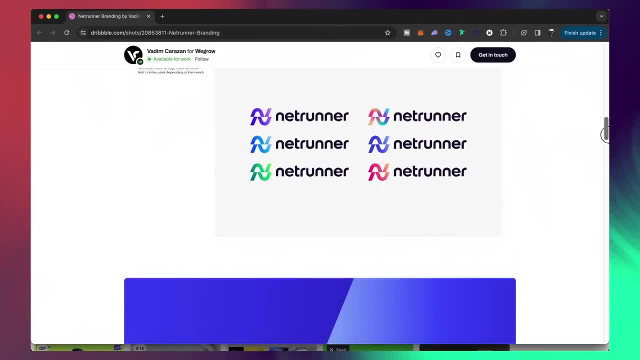 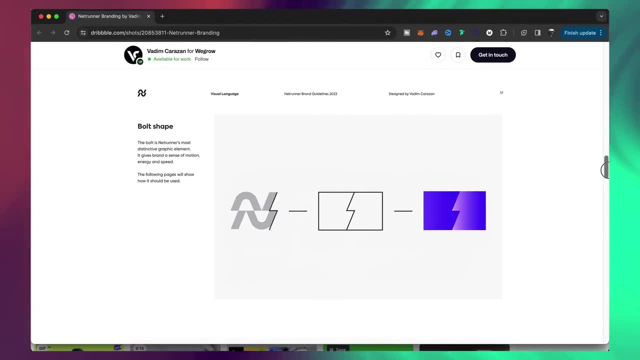 This is what professional designers do. This is what professional graphic design is all about. Consider what emotions this design might want to leverage and evoke, And why does it want to do that. How has a designer made sure this design does leverage emotion? But yeah, this branding project is really neat. 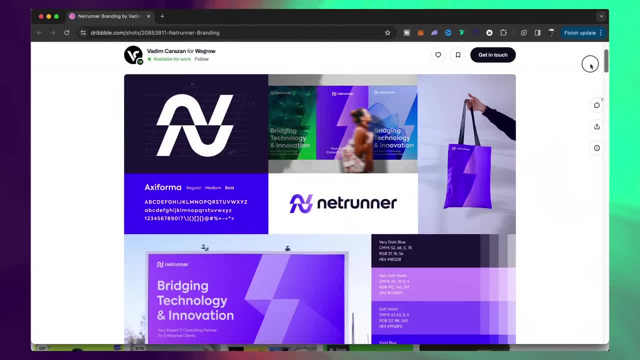 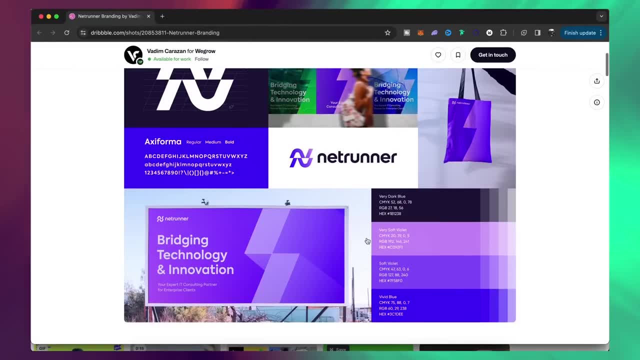 And let's just scroll back up to the top and actually talk about it. So we know the first category is color. But what do you get from the color palette in terms of emotion on this design? So it's mainly blue, purple and a kind of black. 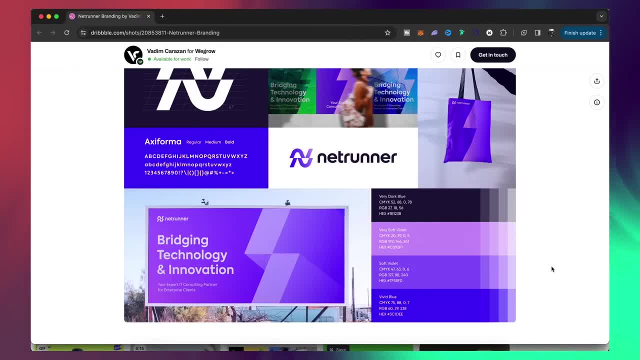 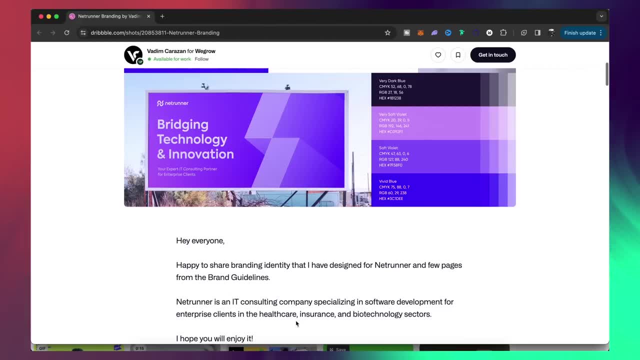 And when considering emotion typically, what do these colors represent? Well, blues and purples do represent a lot of peace, calmness and trust, And that makes a whole lot of sense when you read here that the brand deals with healthcare, insurance and biotech industry sectors. 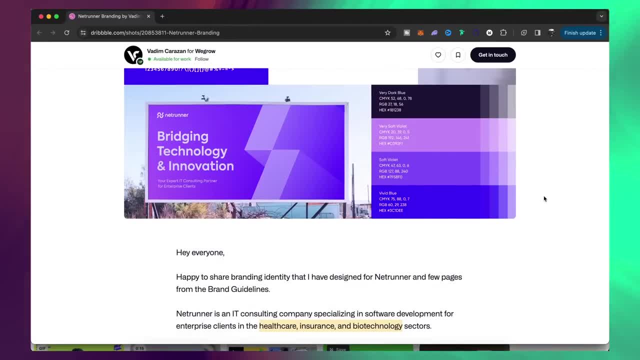 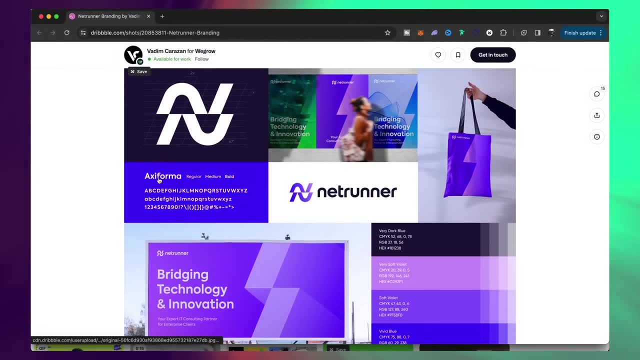 The emotions of peace, calmness and trust are perfect reflections needed in those niches. The color palette here isn't a fluke or just a ruse. It's a random choice. That should be obvious. But hey, let's move on to typography, which might be a bit more complicated. 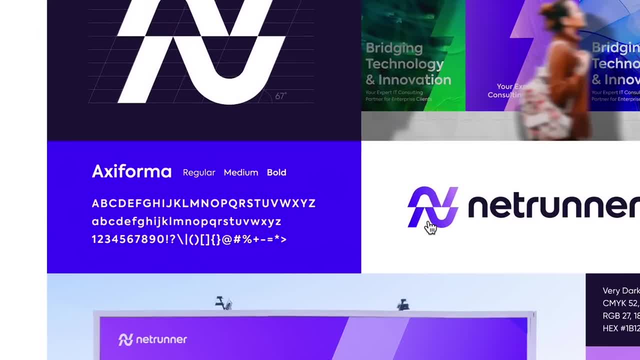 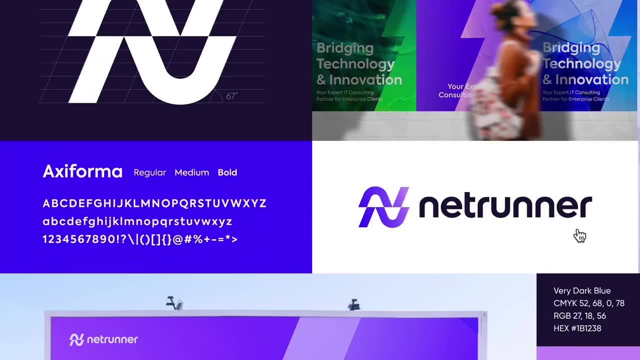 Looking at the typeface, what can we notice here in terms of emotion? For me, firstly, it's the recognition that this is a sans serif font, And it's an ultra sleek sans serif at that. This helps evoke emotions of modernity, which plays into the biotech industry. 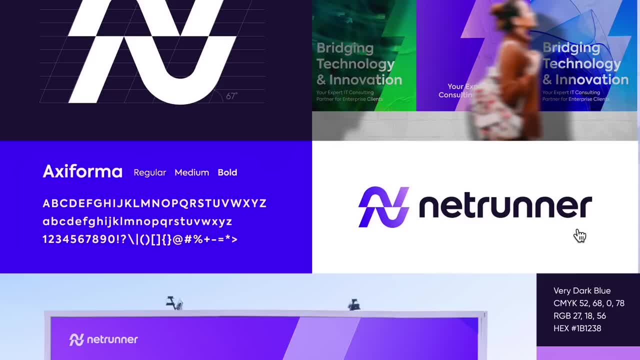 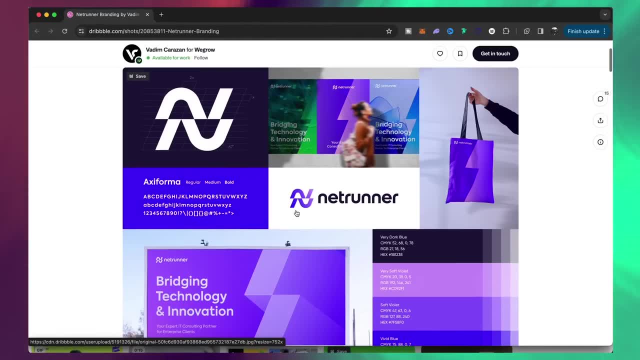 But also it's quite clean, which helps point to healthcare as well. Furthermore, the logo is seen in lowercase. The designer could have easily used uppercase here, But the use of lowercase letters is more informal and more soft, which does help evoke trust. 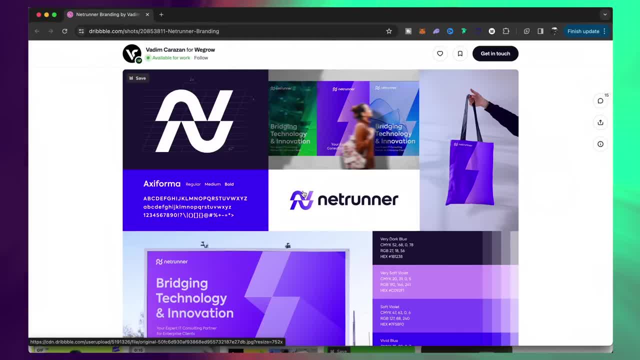 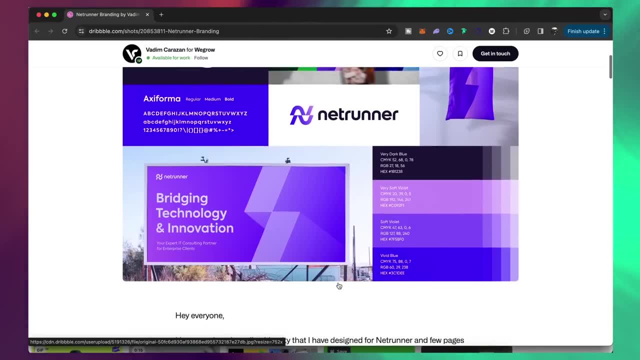 Again, that's great for the insurance industry sector. Also, notice how the clean curves on the typeface mimic the style of the logo. And speaking of the logo, if we look down here we can see the logo is slanted. It's almost italic.